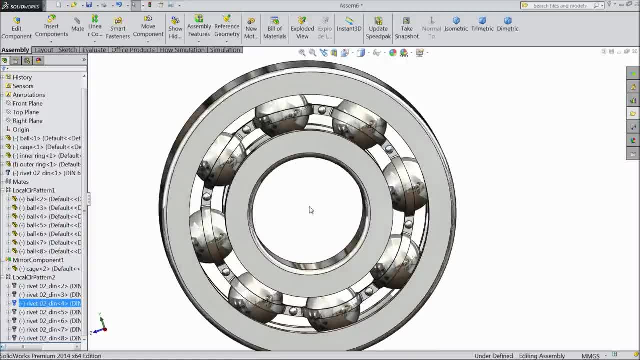 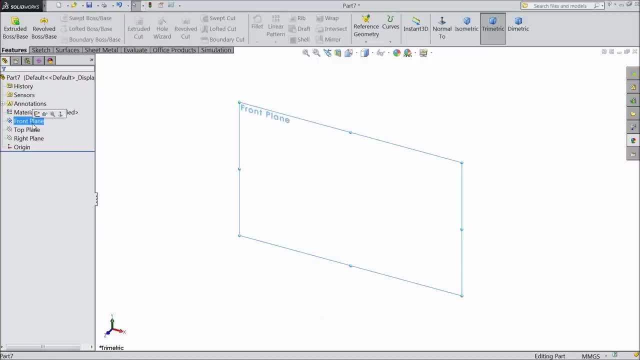 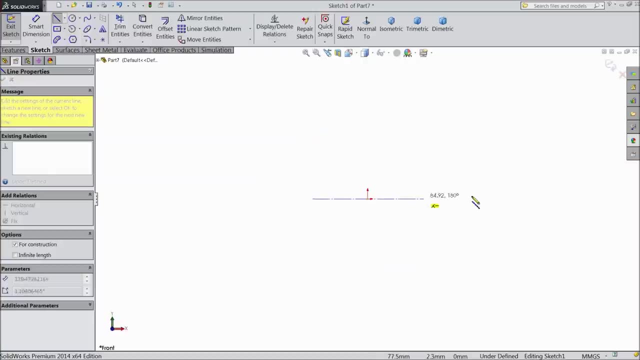 enjoy. So let's start the assembly and design of ball bearing. Now we will sketch first part of ball bearing: inner ring. So let's start. Choose front plane Sketch, Select center line and draw one center line passing through origin. Now choose center rectangle. Okay, 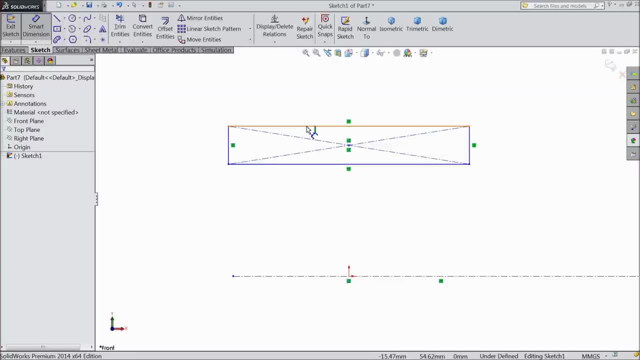 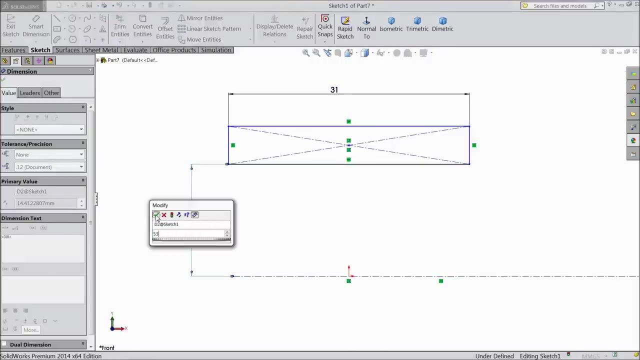 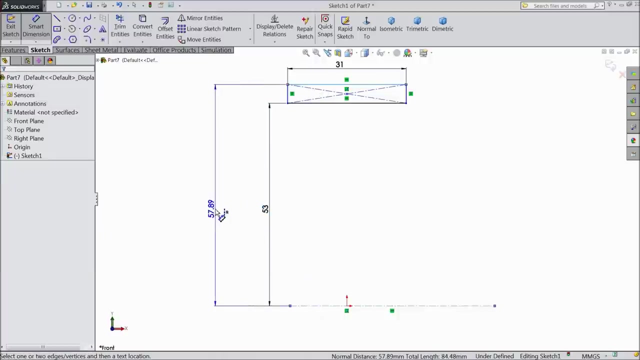 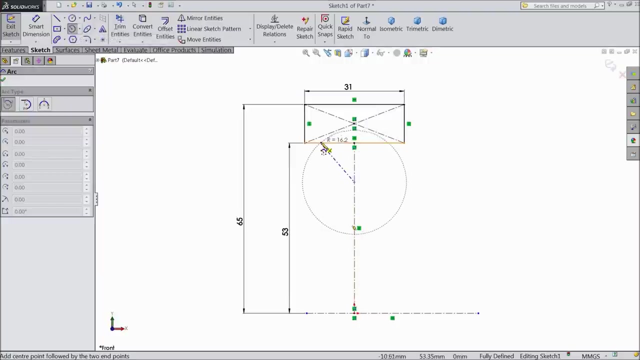 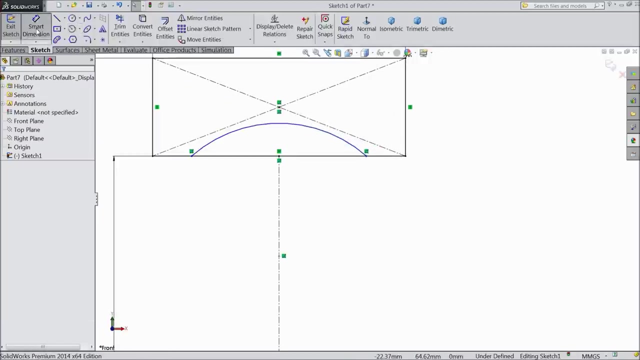 Now we will assign dimensions. Keep the length 31 mm And make this distance 53 mm And this distance 65 mm. Okay, Now select center line and draw one center line to origin. Make sure it is vertical. Now select center point arc. Draw one arc inside the box. Now exit. Choose smart dimension. Select. 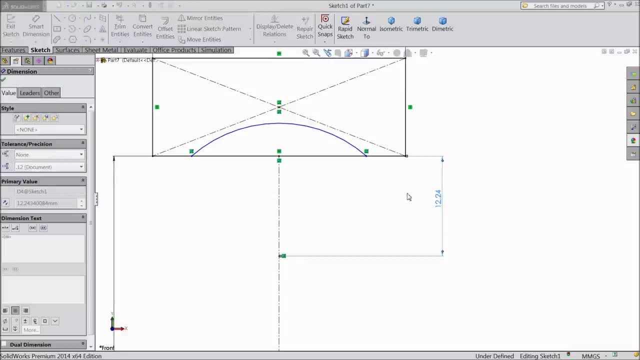 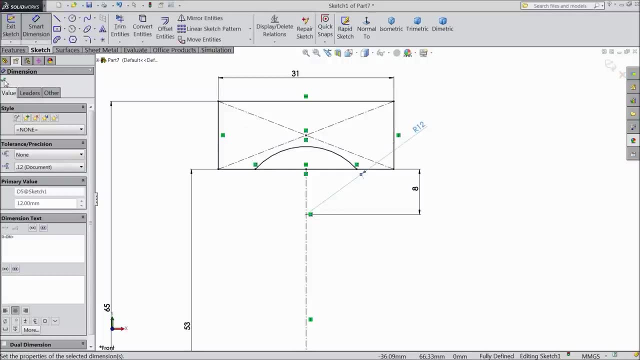 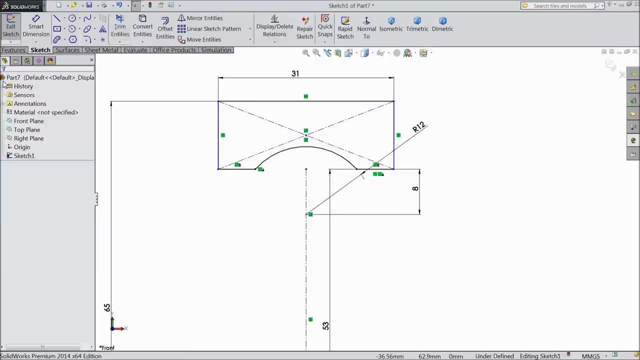 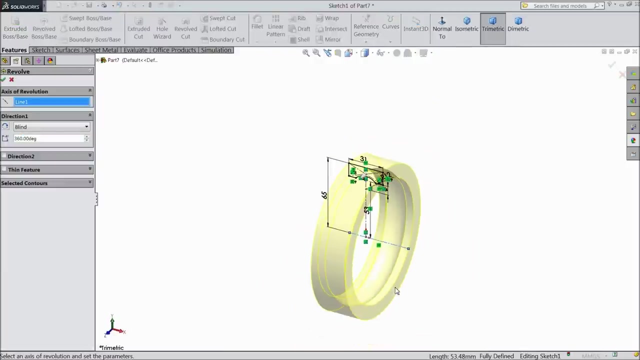 distance from here to this line 8 mm and keep the radius 12 mm. Ok, Now choose trim and trim inside, Inside. Ok, Now select this side line and this side line. Make equal, Equal relation. Ok Now revolve boss base. Select this as a axis. Ok, Select chamfer, Select. 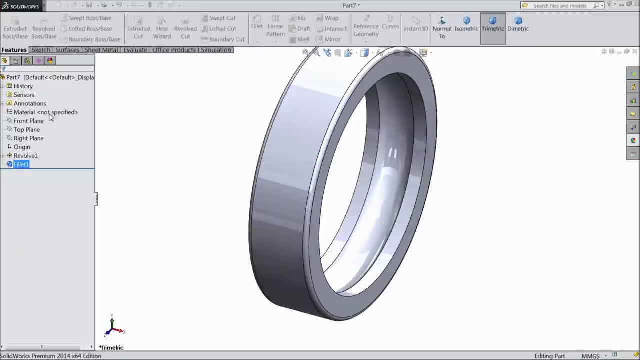 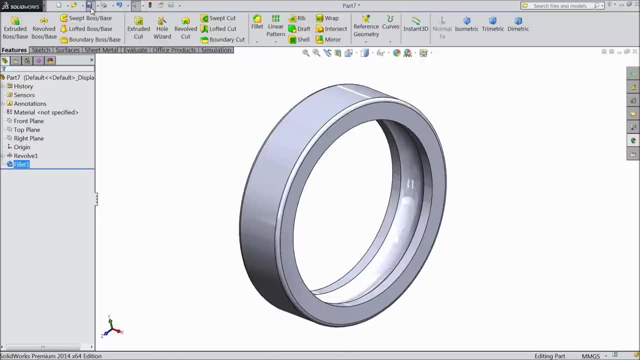 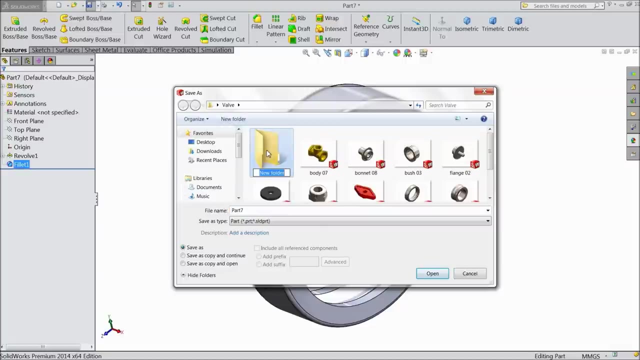 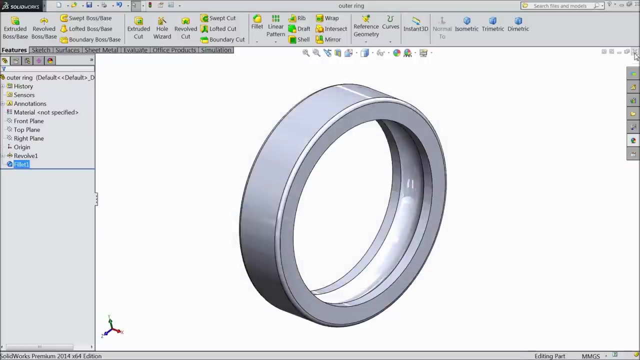 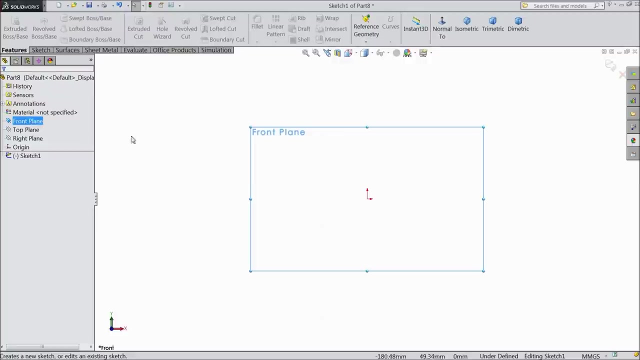 2.1 and select this face. Ok, Now, inner outer ring is ready. Now save it. New folder Ball bearing Right outer ring. Ok, Now we will make second part, inner ring. So choose front plane Sketch, Select center line and draw one center line. 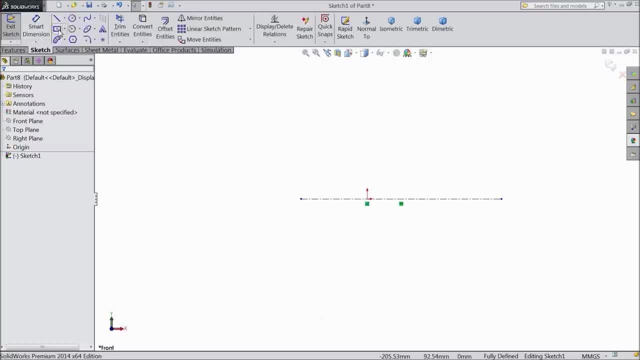 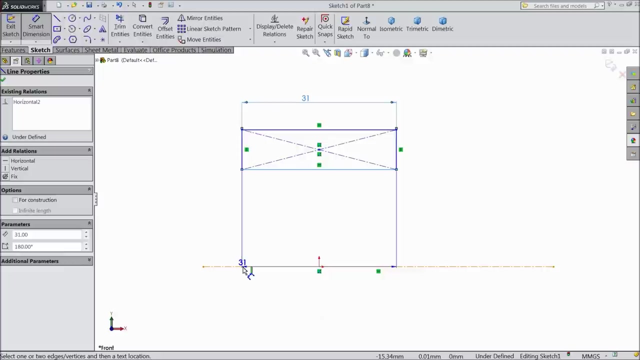 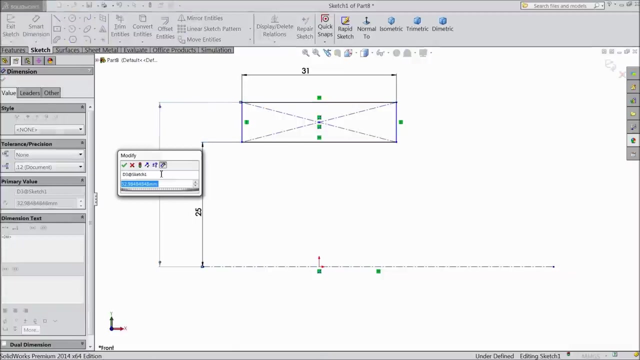 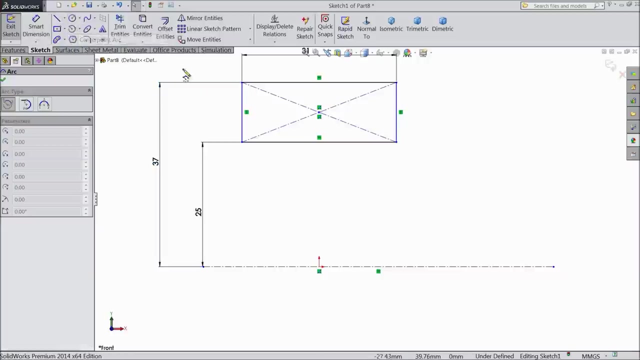 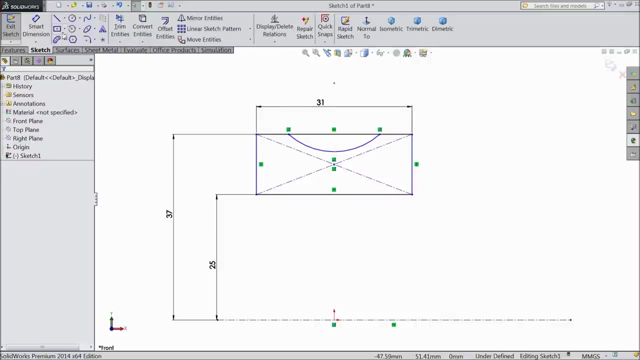 Horizontal line. Ok, Now select center rectangle. Draw one rectangle like this: Ok, Now we will assign dimension. Assign 31 mm, Distance from here to this line 25 mm and outer line 37 mm. Ok, Now select center point arc And draw one arc. Now exit. Select one center line. Connect. 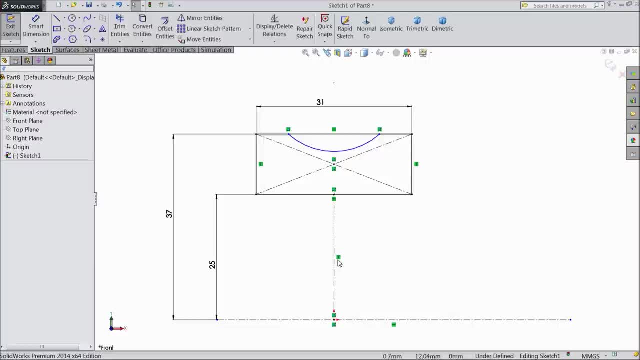 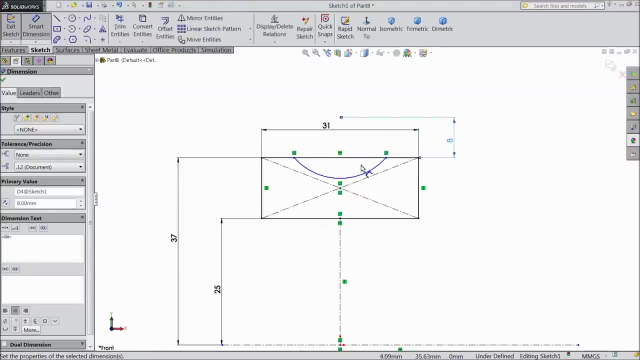 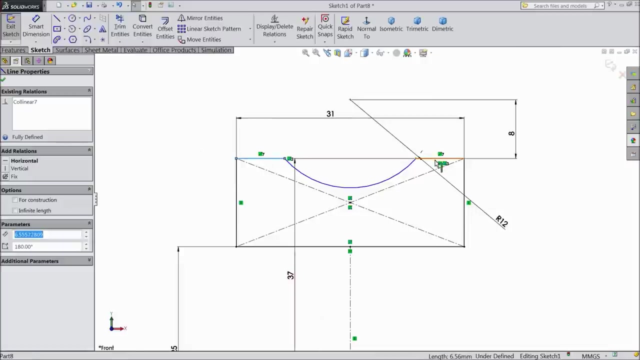 from origin point. Make sure it is vertical. Ok, Now again choose distance from here to this line: 8 mm And radius: keep 12 mm. Ok, Choose trim entities and trim inside portion. Ok, Now select this outside line. Both side, Make relation equal. Ok, Now choose fillet. 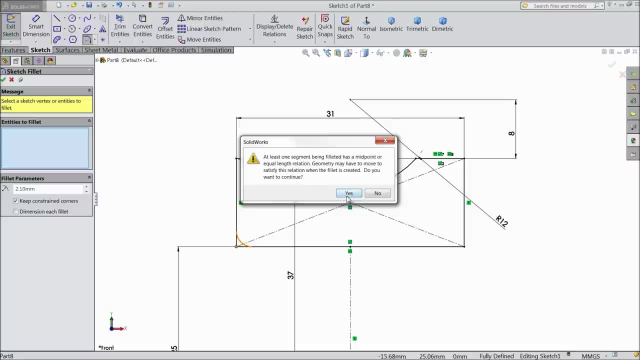 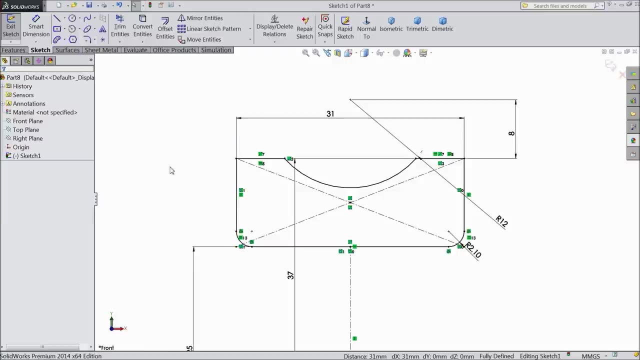 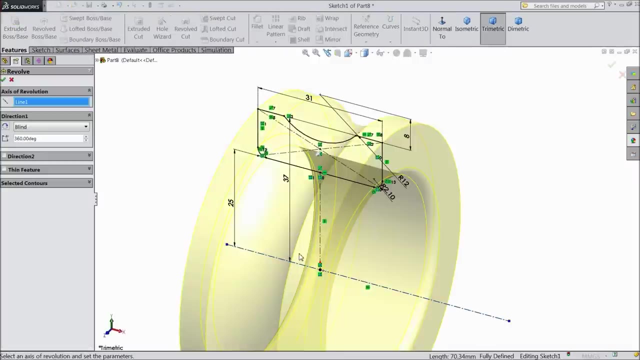 Set 2.1mm and name this as the face. Ok, Now our flow. I am rotating circleacam intoaddline Now. our structure is fully defined. Now go to features. Select revolve boss base. OK Now. 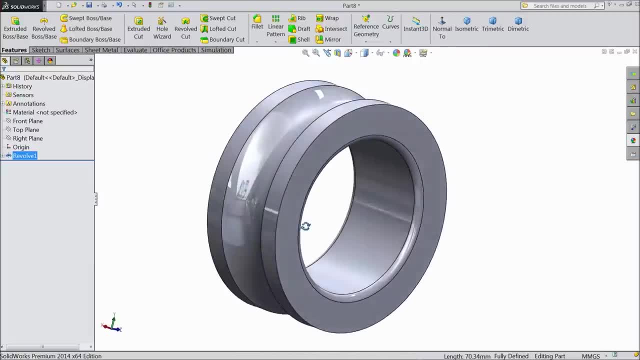 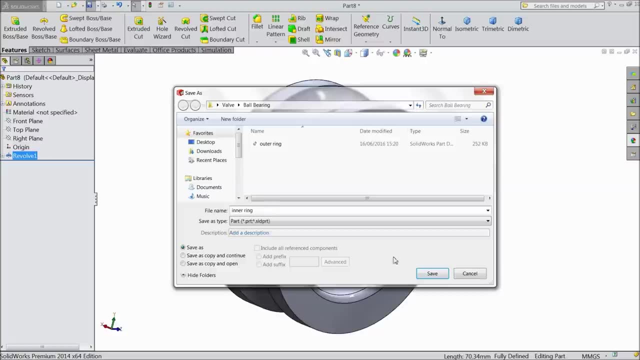 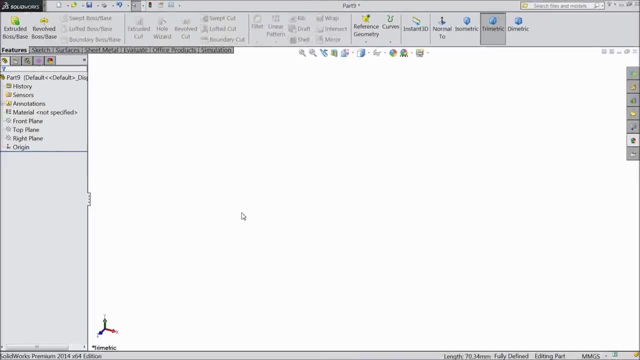 this inner inner ring is ready. Now save it. Continueults. section of main line is done, And now next, next. OK, Then this is the original. now This is kind of rectangular cylinder in this inner ring. now go for next part. now we will sketch third part of ball bearing ball. so 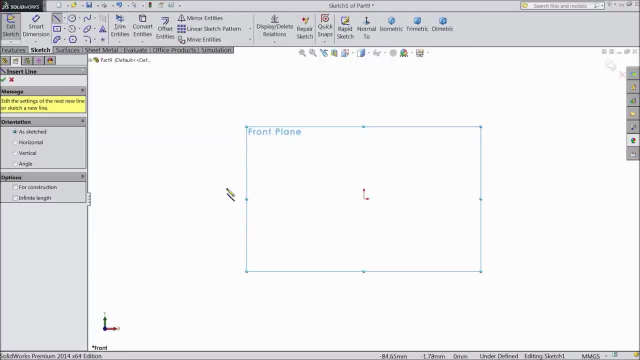 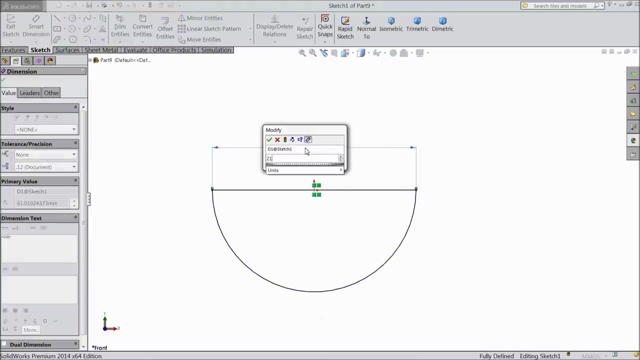 choose front plane sketch, select line and draw on line. just go back and draw a half circle. okay, now exit from the line. just select this center of the line, shift key, origin point and here choose, make coincident, now it is center. choose smart dimension and keep the length 12 mm. 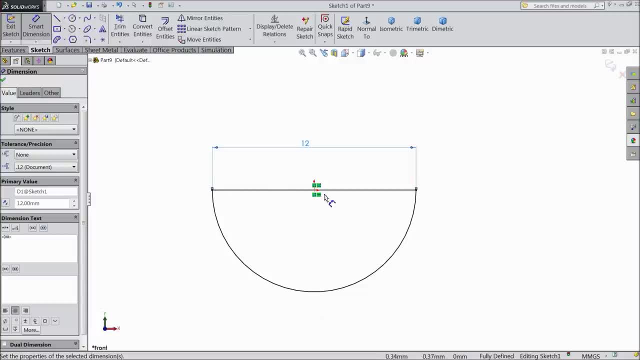 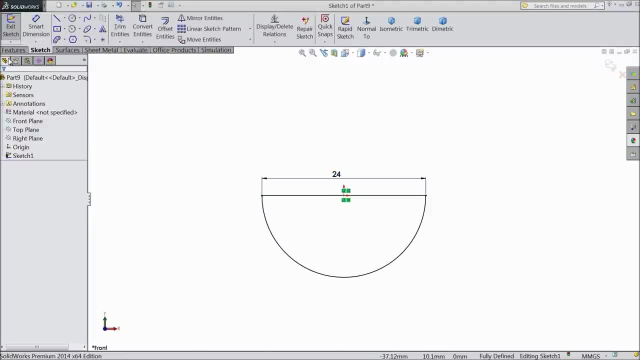 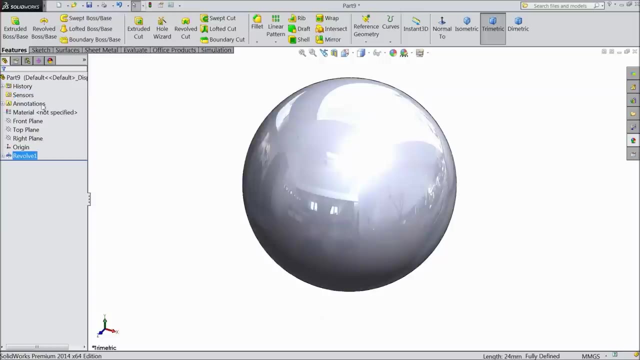 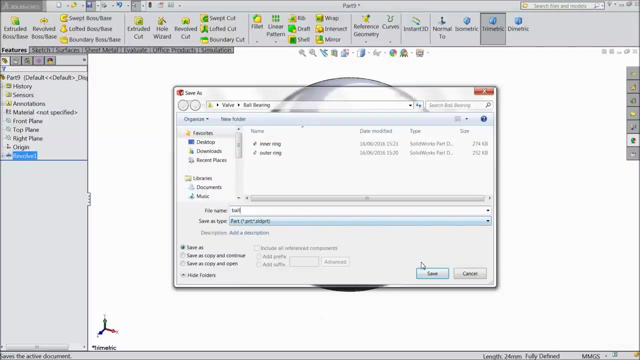 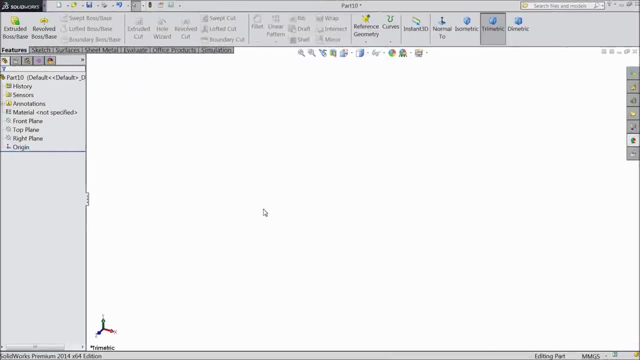 12 mm, okay or no? keep 24 mm, okay. now choose revolve boss base. select this. okay. now, save it ball. now, this is the ball we saved. now go for another part. now we are going to sketch key. now we are going to sketch key. now we are going to sketch key. 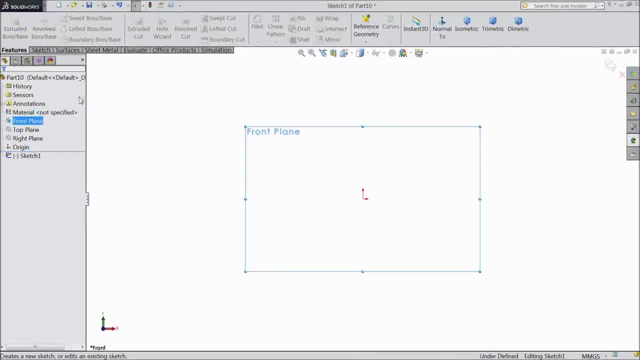 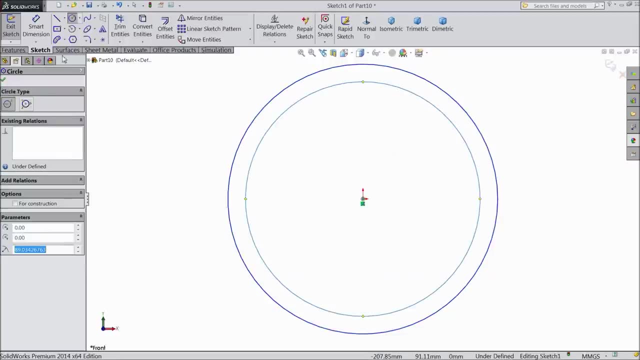 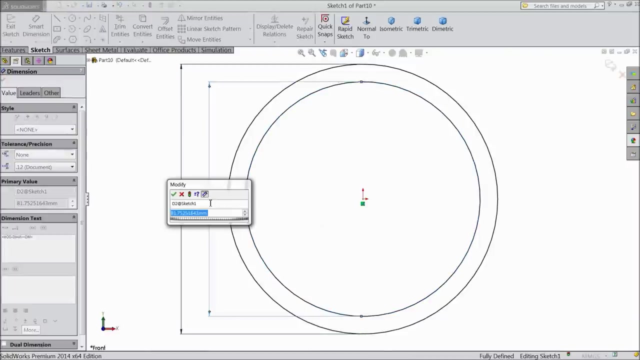 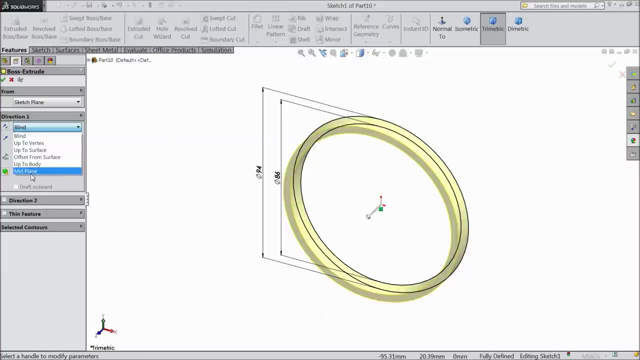 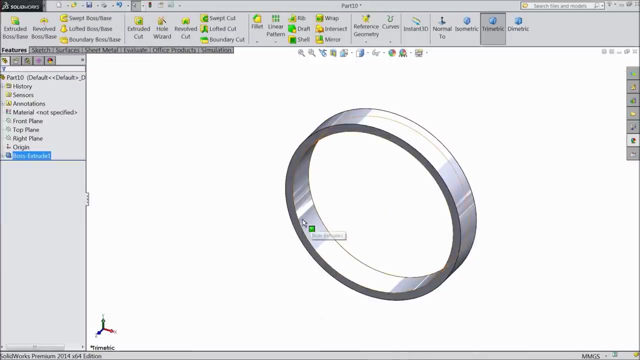 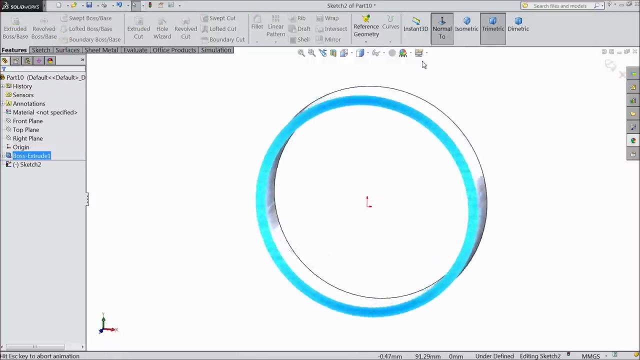 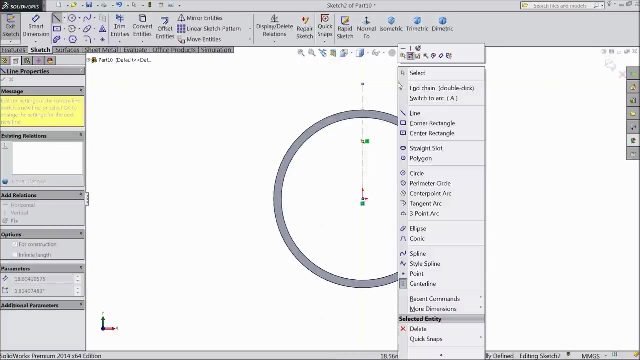 for ball bearing. so choose front plane. sketch. draw two circles from origin point. now assign diameter outer 194 mm and inside 86 mm. okay, select extrude boss base. choose mid plane. keep width 16 mm. okay, James, now select this face. he will sketch set normal. 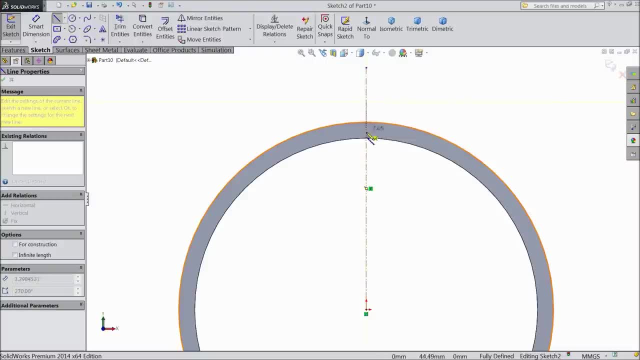 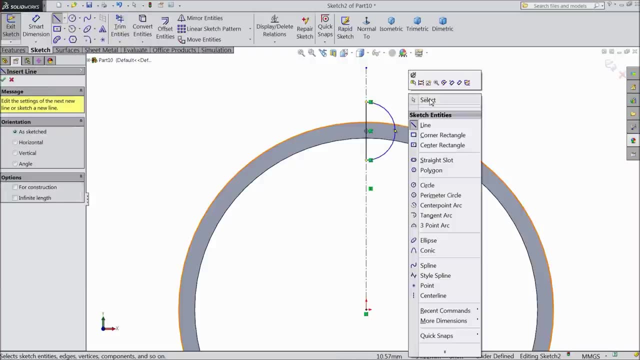 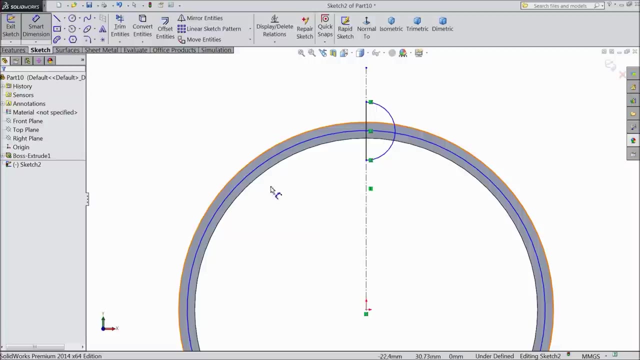 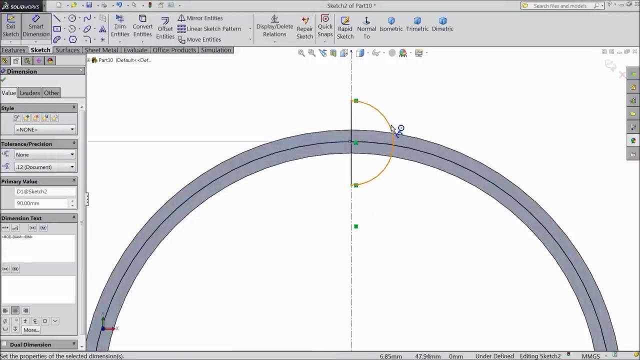 choose centerline and draw one. the centerline exit. select line and draw a line. go back and draw a half circle. exit from the line. then choose circular. then select standard straight line circle, draw one circle up to mid and assign diameter 90 mm. and ok, now select the center. 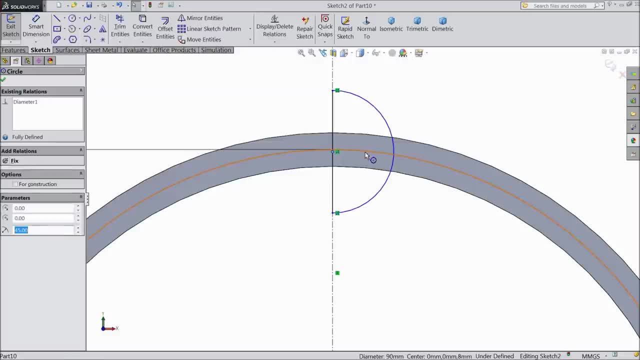 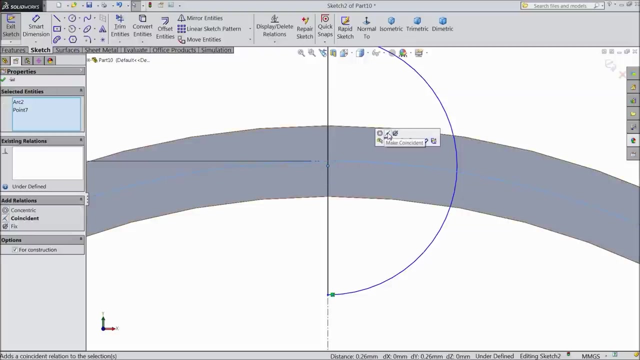 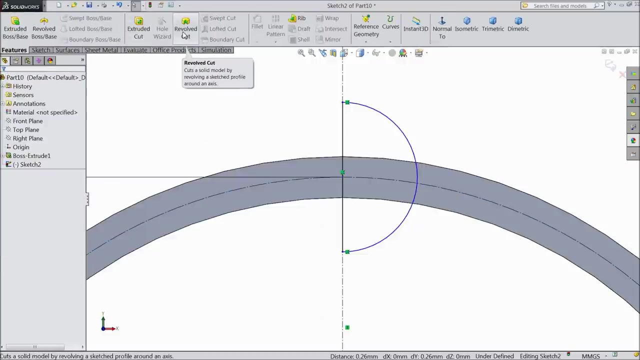 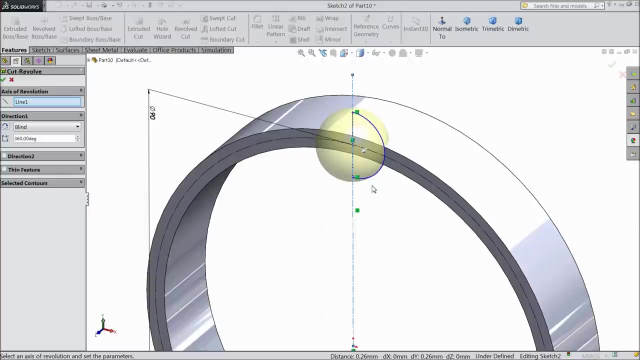 point of this line and select this diameter. first select this for construction. now center point and this line: click here relation. make coincident: ok, delete this relation. now choose this point and this point. make coincide: now it is coincide with this. ok, now select revolve cut. see, is going to cut from inside. select, ok, now choose fillet. 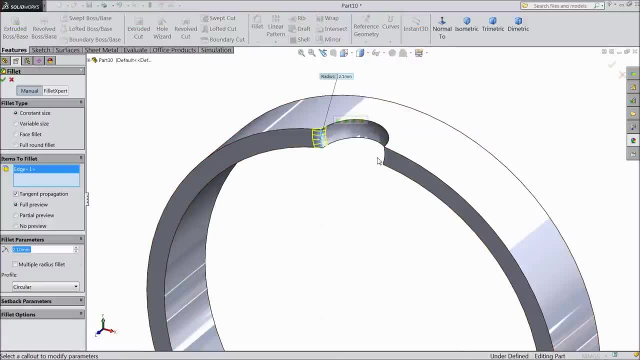 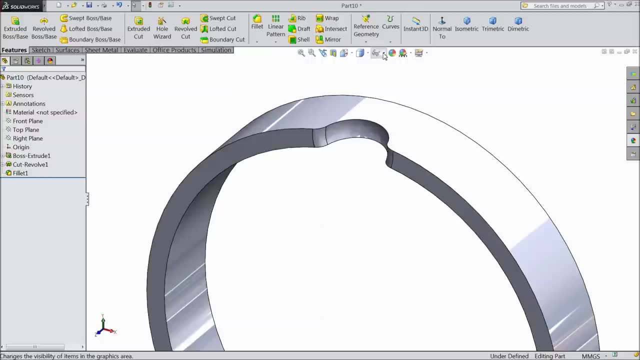 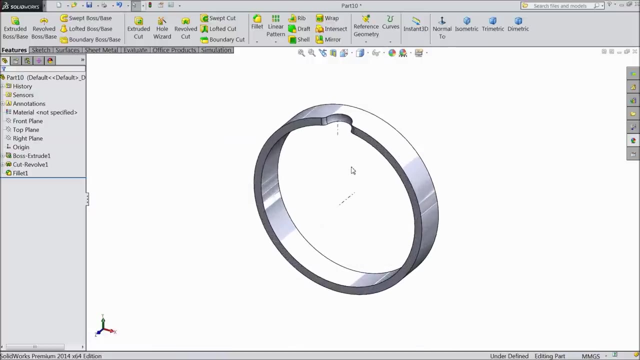 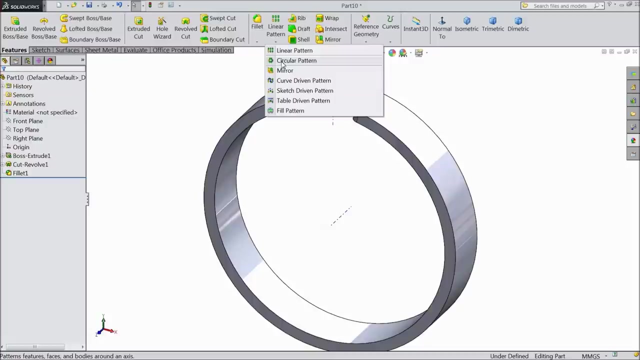 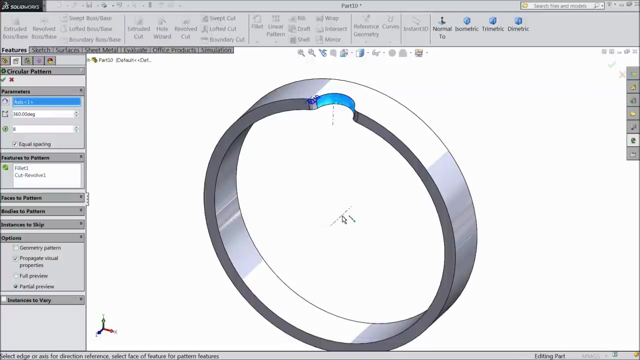 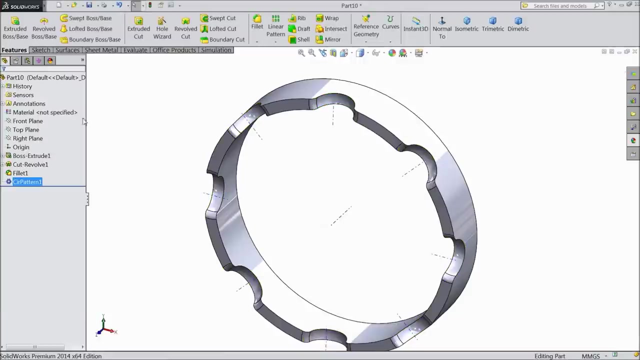 2.1 mm and select both the corners. ok, now here show item and click temporary axis. now see temporary axis are visible. now choose circular pattern. select this, cut out and this. choose this line as a axis. we want 8 numbers, 360 degree, equal spacing. ok, now see the half portion is created. now select 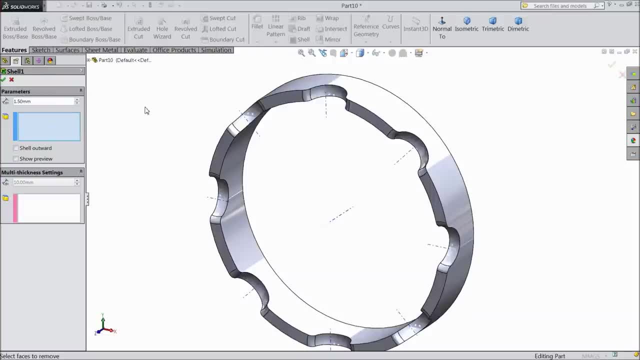 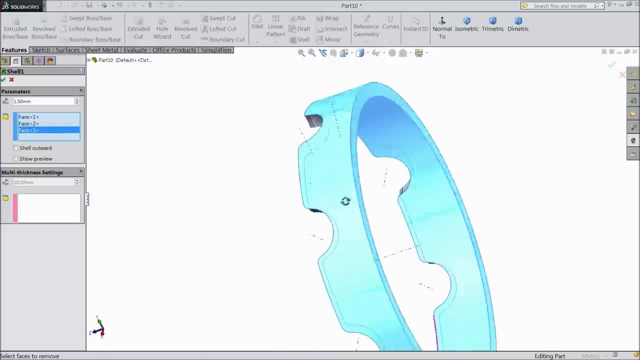 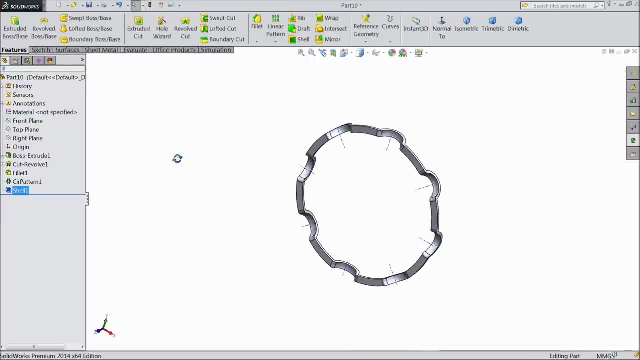 shell. keep thickness 1.5 mm and select this outer face, back face and inside face, only remaining this outside face, 1.5 mm. ok, see, now do one thing: sketch, click on sketch. select this first flow, advantages and side thesis. like already pracy, select here. show this looking. select this portion. now our circle is looking small. 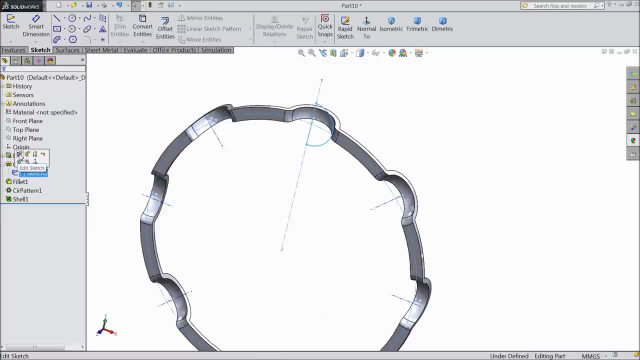 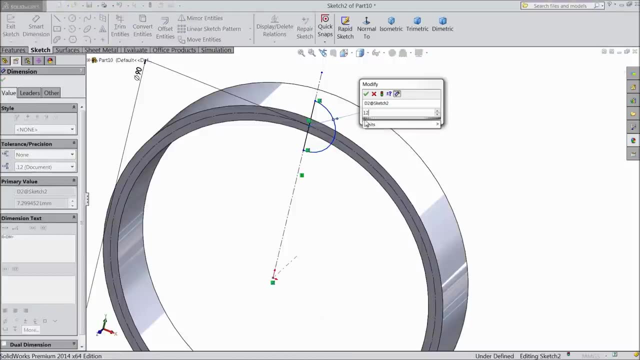 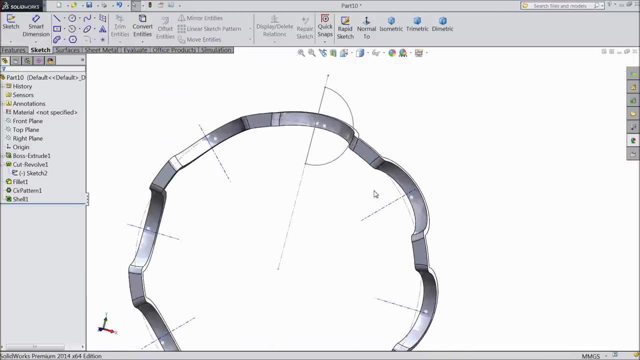 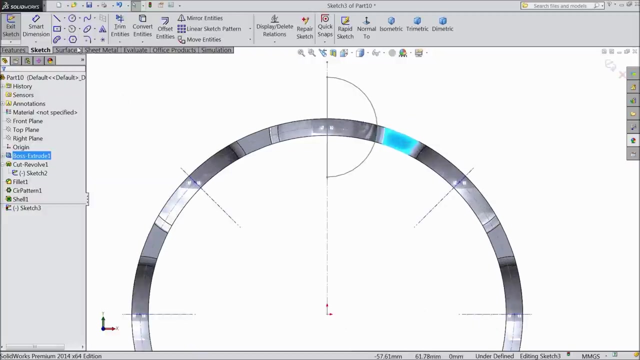 so just select edit sketch. choose smart dimension and select this radius. keep this radius 12 mm. now exit. ok, now our sketch looking perfect. select this face sketch: normal. now choose a center line and draw one line from here to this circle. select. 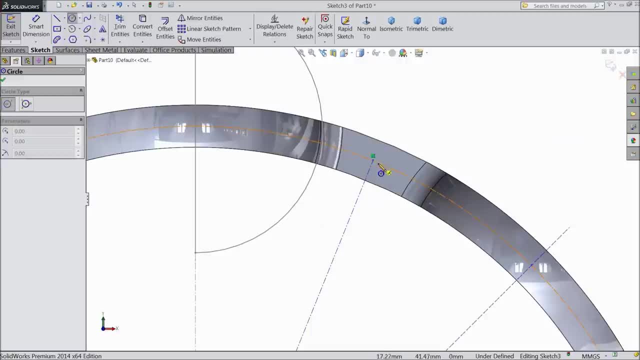 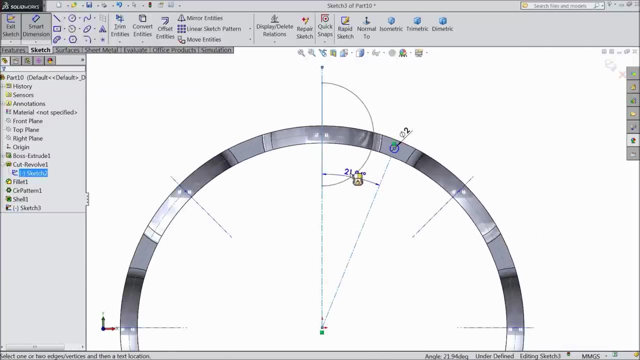 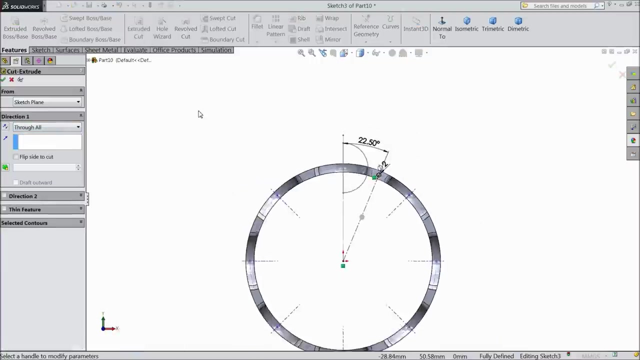 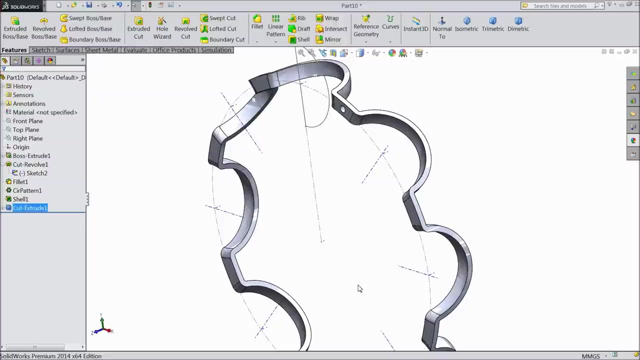 this exit. choose circle and draw one circle here and assign diameter: 2 mm. ok, now select. now assign 360 by 16 mm. this is our angle. ok, select extruded cut and choose through. all is going to cut. ok, now select circular pattern. choose this. 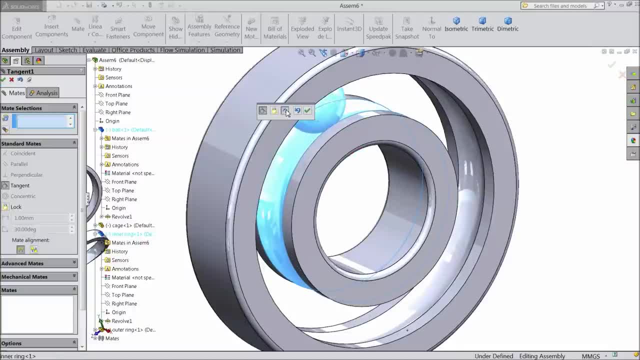 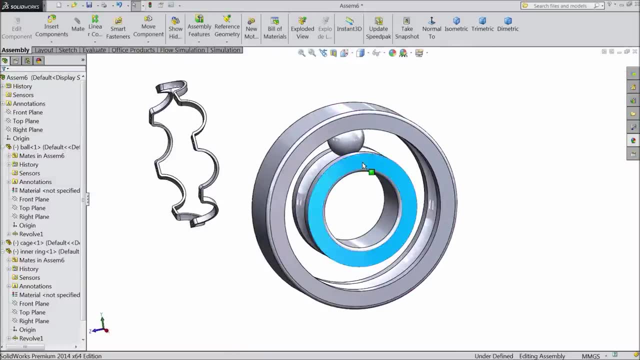 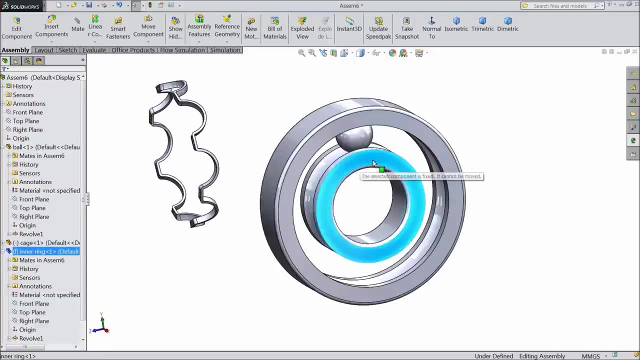 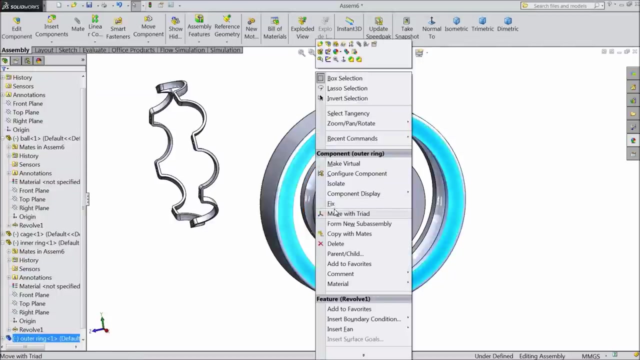 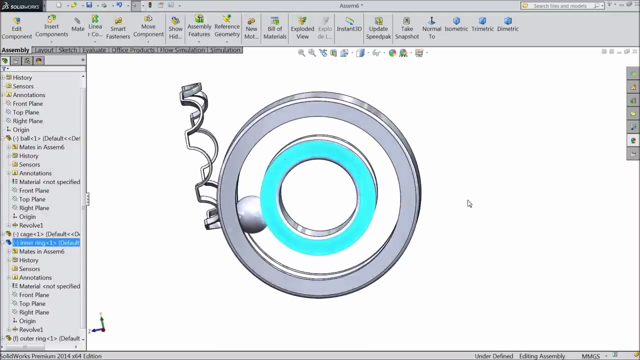 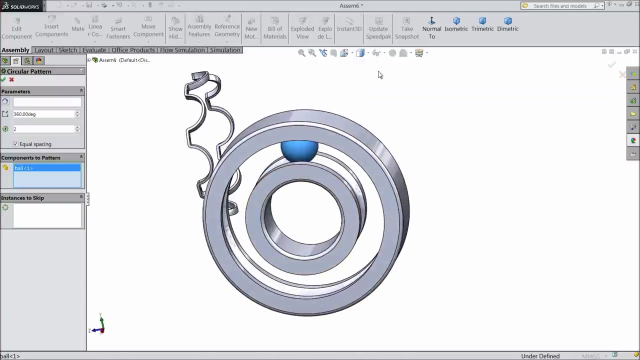 inside: select flip mat. ok, ok, now see this one. select fixed now this. now make it float. select this outside: fix. now. see it is rotating inside. now we will make circular component. now we will make circular component. now we will make circular component. choose ball, select temporary axis and. 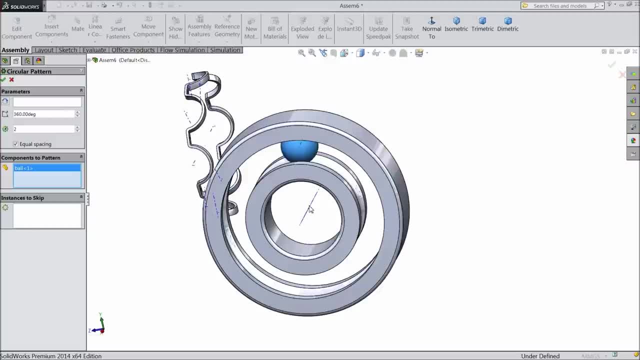 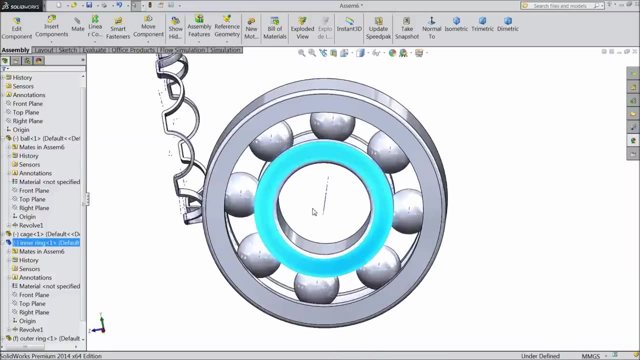 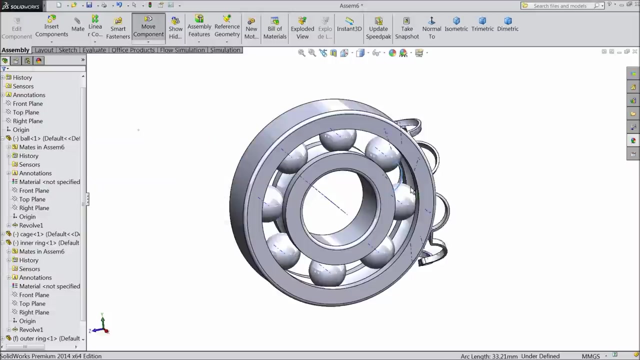 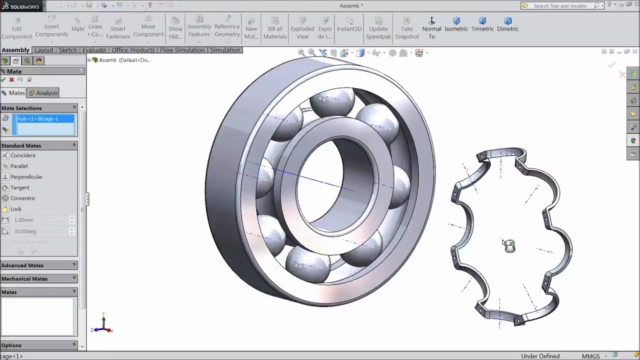 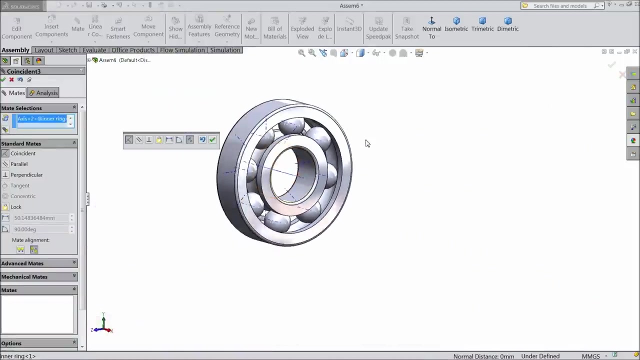 select here this axis and make it number of balls. ok, now see it is rotating, rotating 8 number of balls. now bring this part here, choose matte, select this center. line this here very small, looking here- and select this center, choose ok, drag it this. 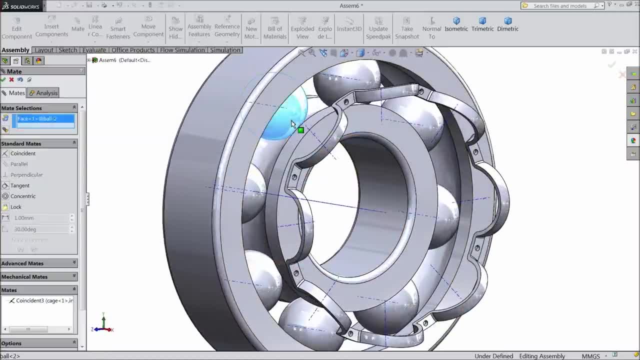 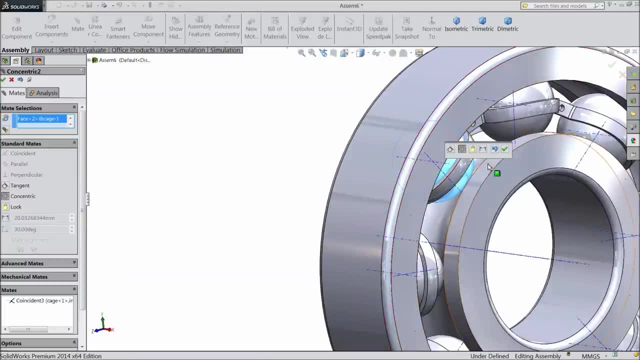 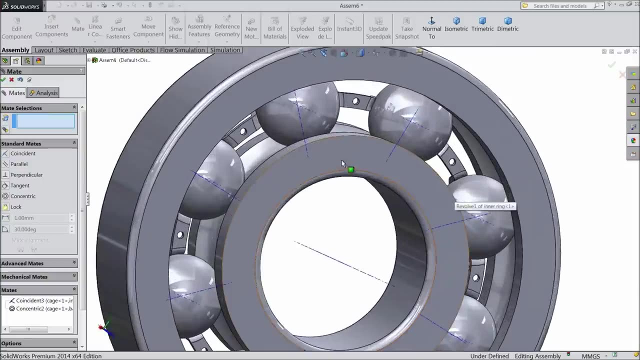 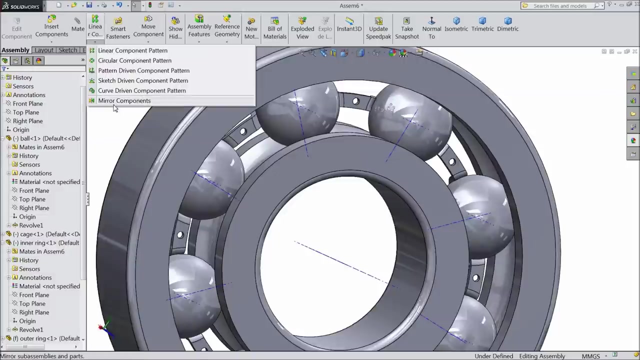 side. now select ball and this inside face. see, it is fixed with here. now we will make reverse, so just go to back reverse. ok, now we want to make mirror for this, so select mirror component. select this face. we want to mirror of this, so select mirror of this. 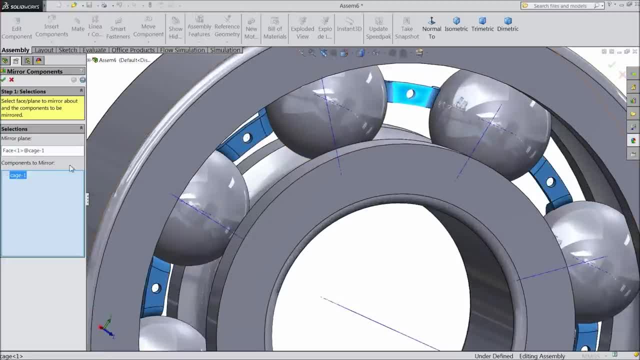 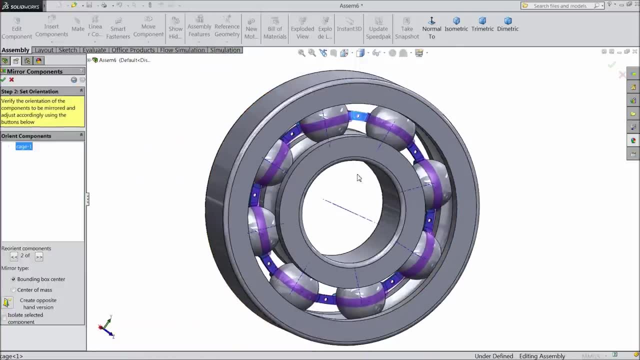 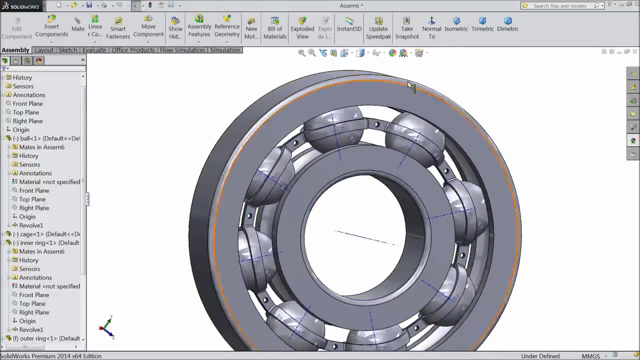 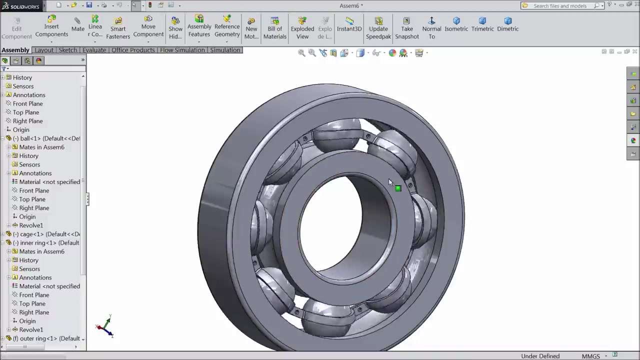 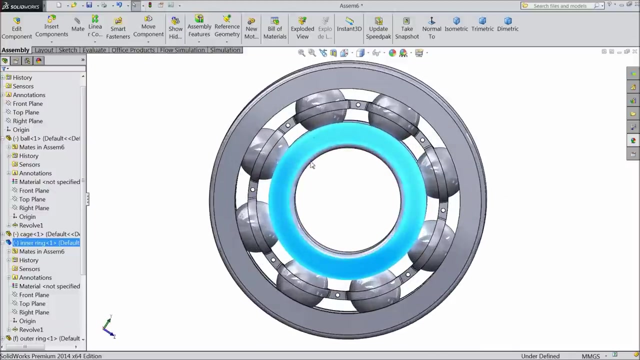 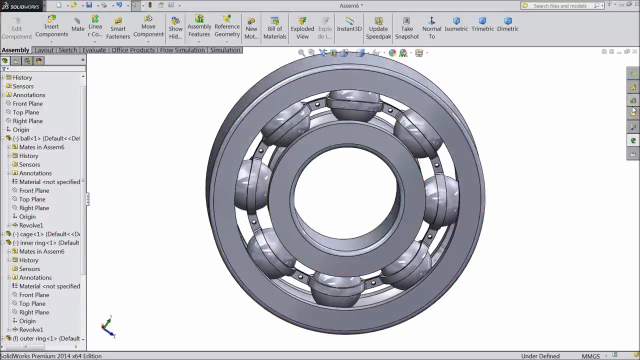 mirror on this face and choose this body. ok, now here one key. select next. now see it's showing your component going to be. mirror this side, choose. ok now. hide temporary axis. now see it is rotating. Now here, ball bearing is ready. now only we have to fix some rivet. so go to toolbox.